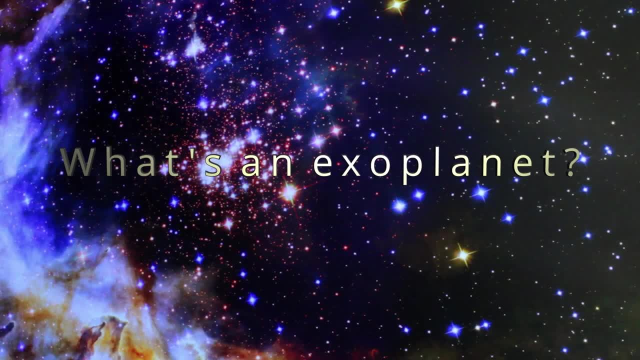 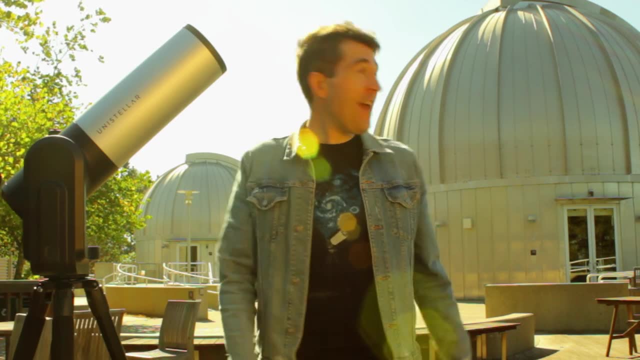 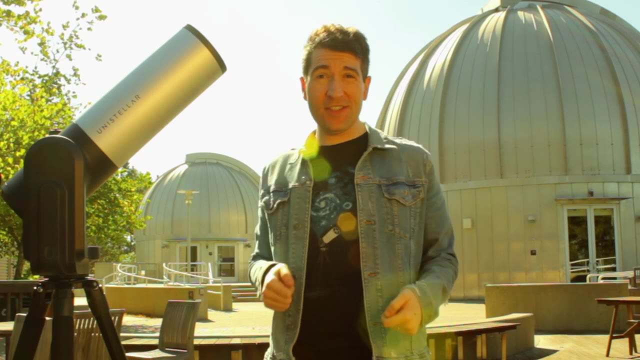 Well, what's a planet? I'm here at the Chabot Space and Science Center in Oakland, California, And behind me on the observation deck, astronomers use these telescopes to show the public the planets of our solar system. What do you think a planet is? What do you know about the planets in our solar system? 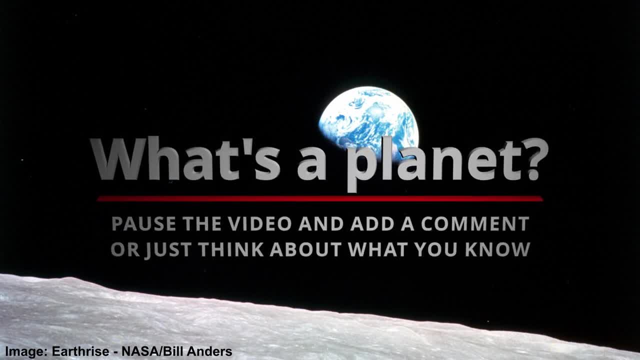 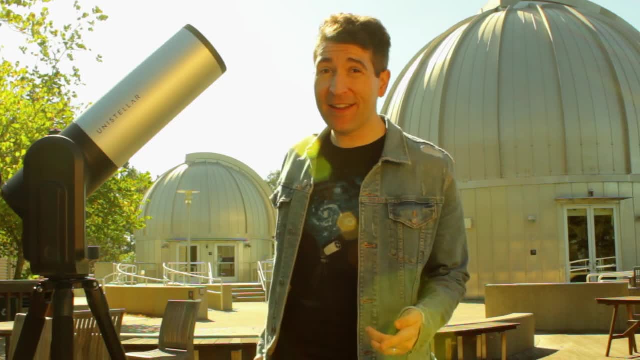 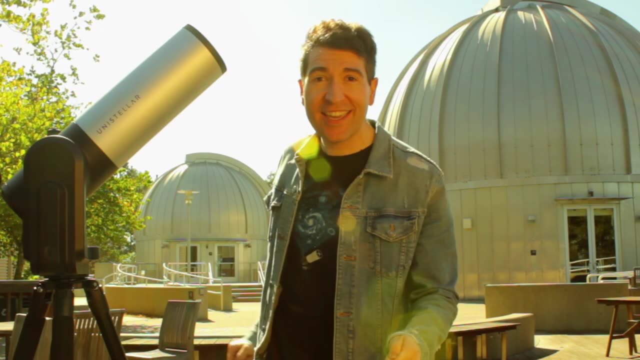 Pause the video and write a comment to tell us what you think. So what are planets? They're places where things happen, And on some of them, some really interesting things happen, Like here on Earth. life has evolved to the point where it started speaking to each other and asking interesting questions, like 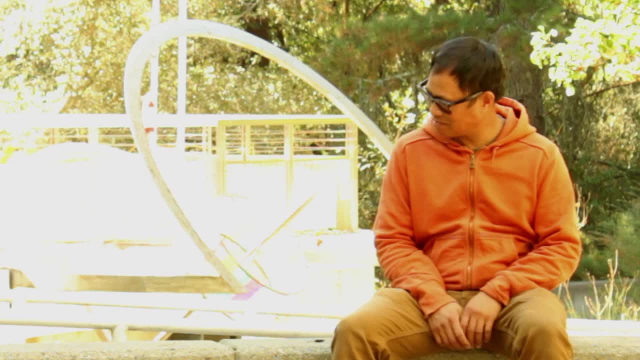 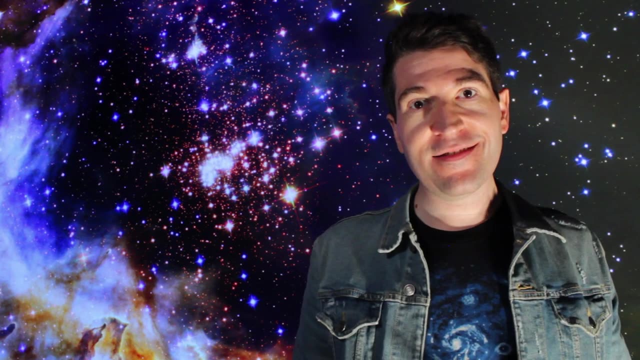 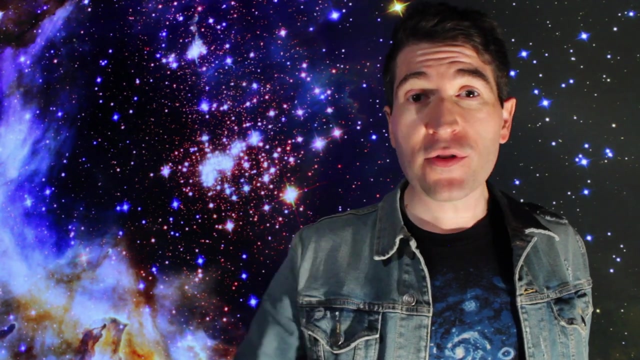 Eric, what's an exoplanet? Astronomers define an exoplanet as a planet that orbits around another star other than our own sun, And there are hundreds of billions of stars just in our own Milky Way galaxy, And we now know through telescope observations of thousands of confirmed exoplanets. 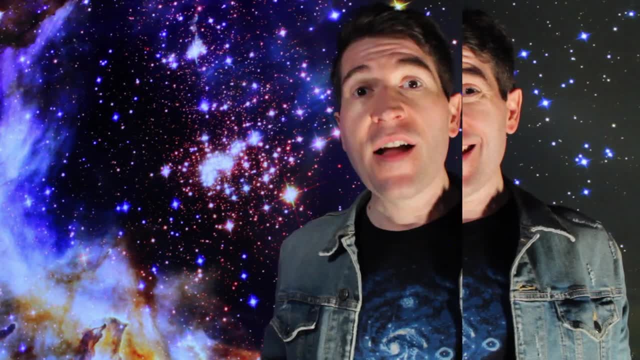 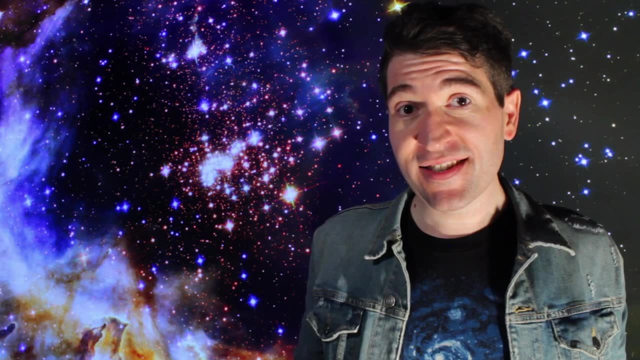 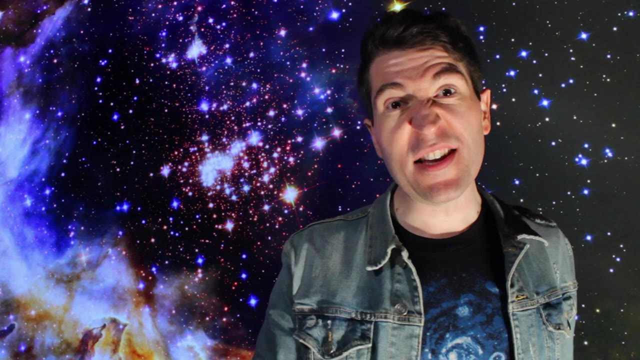 And from that information we can estimate that there's about one exoplanet per star in our galaxy. That's a lot of places, A lot of possibilities for some very interesting things to happen, And there's a diversity of worlds too- Giant gas planets. 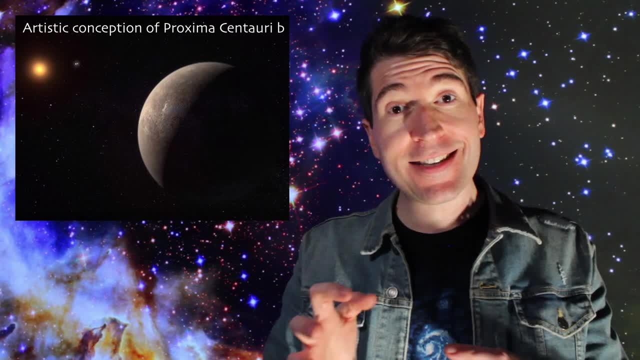 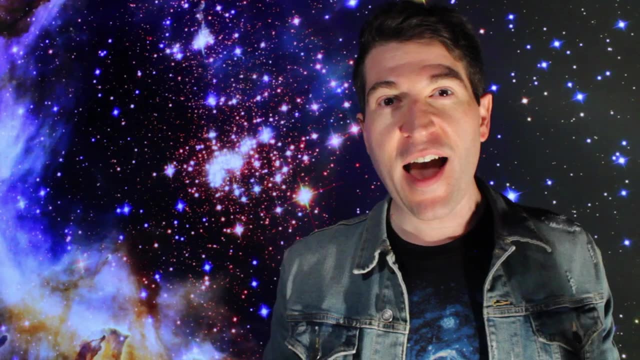 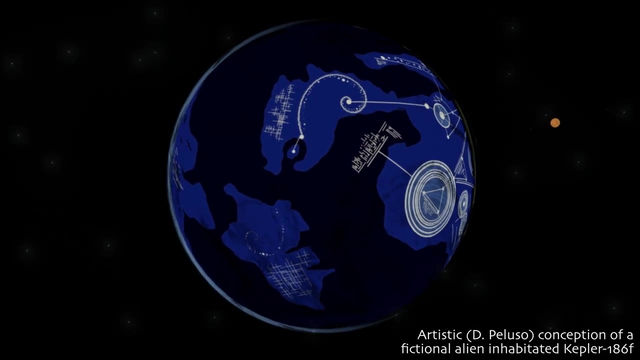 Small, rocky, terrestrial worlds, Estimates of tens of billions of planets similar to Earth, And astronomers even have planets that they call super-Earths. Imagine this. Imagine just on one of those exoplanets, life has evolved to be curious and to ask questions such as. 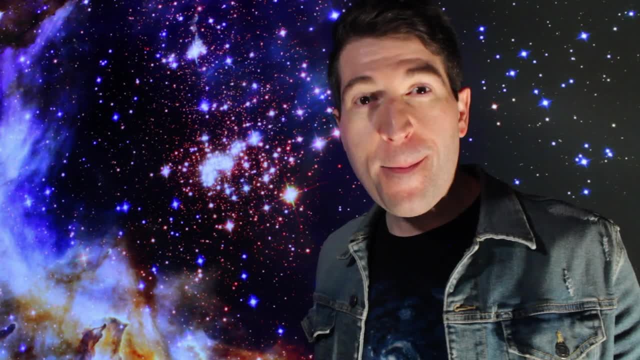 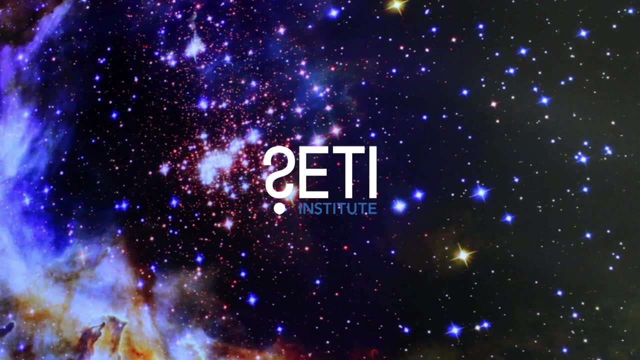 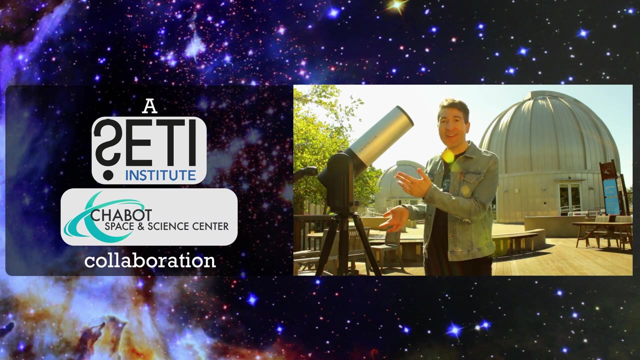 Are we alone? Maybe they're looking for exoplanets, Maybe they're looking for us. I hope you enjoyed the video. If you noticed, there's this interesting looking telescope to my right, Or is it to my left, I don't know.